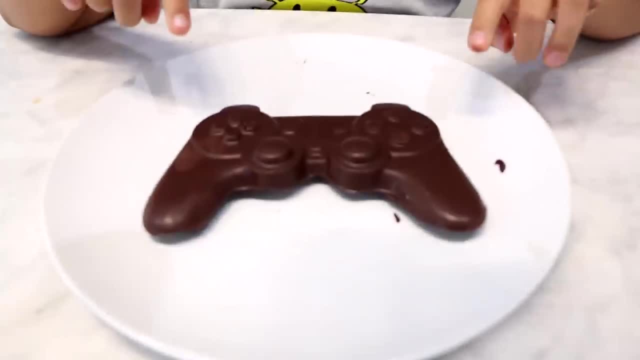 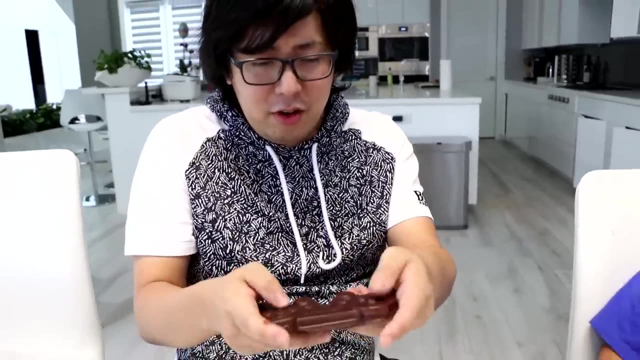 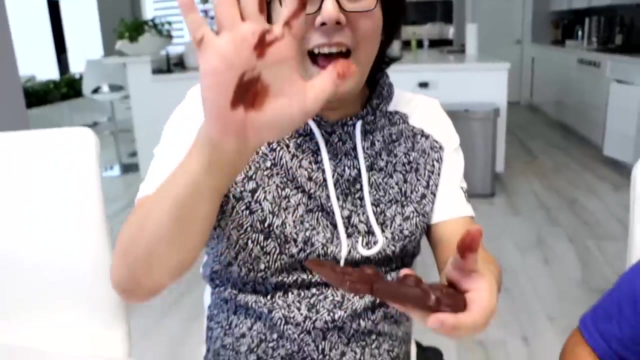 Look guys, my chocolate remote is done. The chocolate piece physically changed from this to this. Can I actually use it? Yeah, For my gaming. Are you sure? I don't think the buttons are working. It's melting. Welcome to Ryan's World. 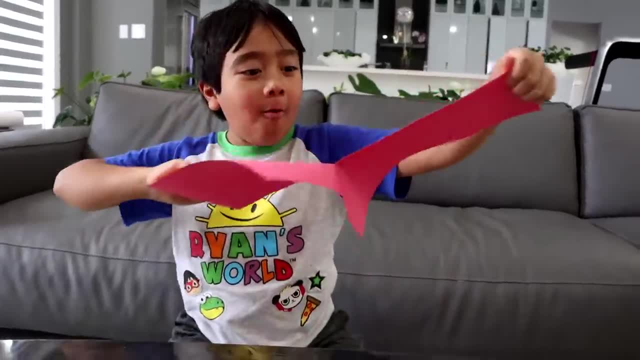 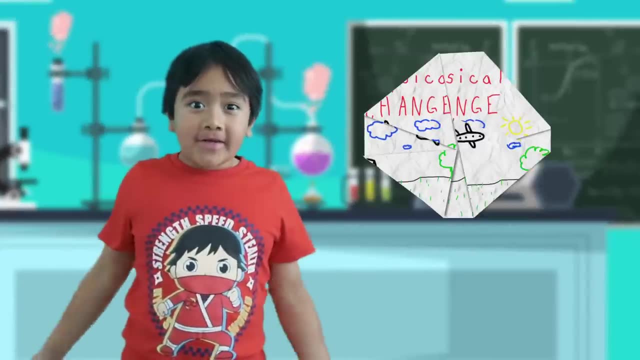 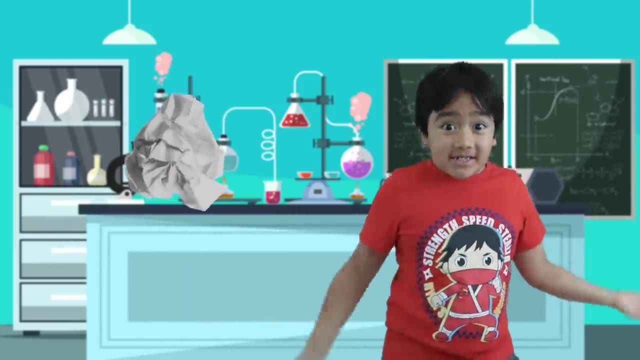 Hey guys, I'm ripping paper. Did you know that ripping paper is a physical change? A physical change is when nothing new is formed or created. You can change the state, size or even how it looks, but it's still the same. 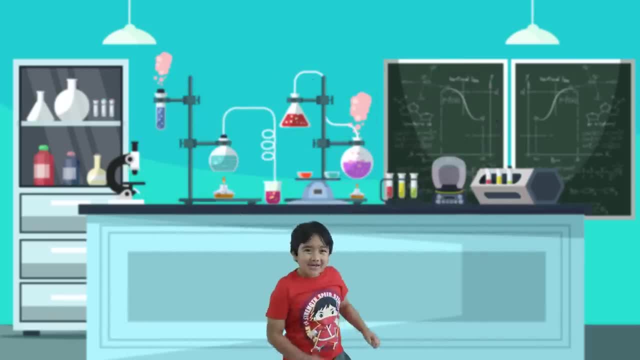 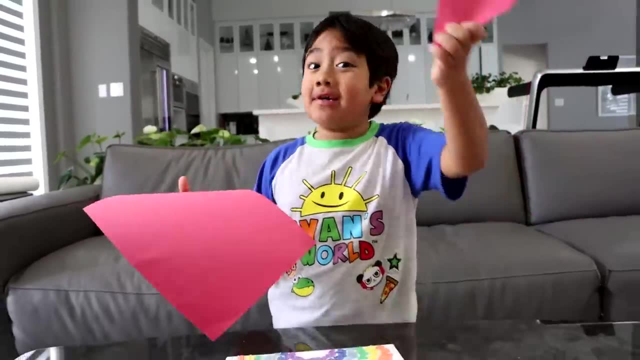 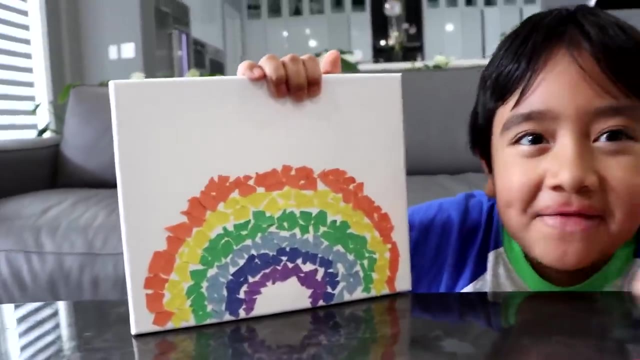 It just looks different. Physical change. Ripping paper is a physical change because this and this are both paper. I didn't create anything new because this is still paper. I tear up a bunch of paper to make a rainbow, So let's finish it. 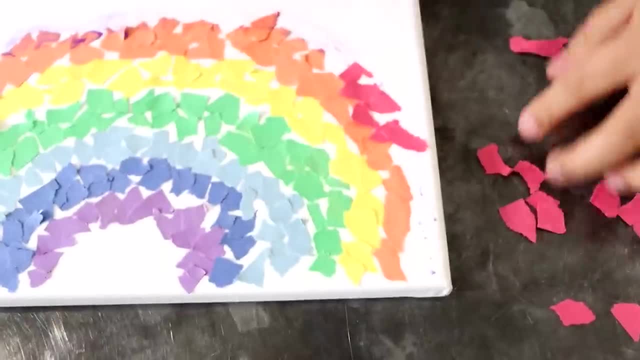 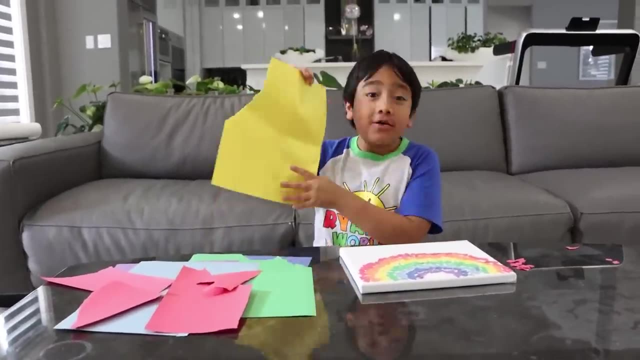 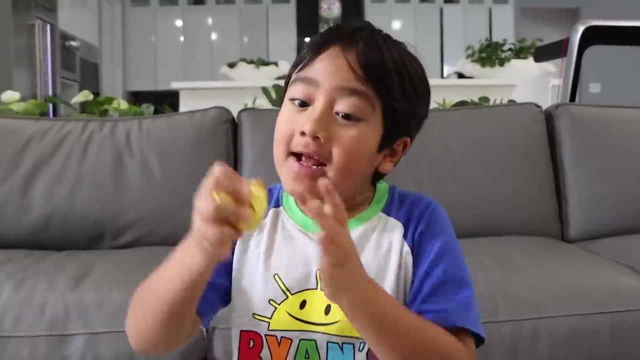 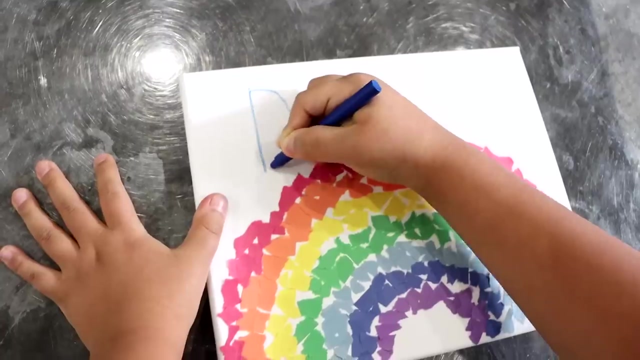 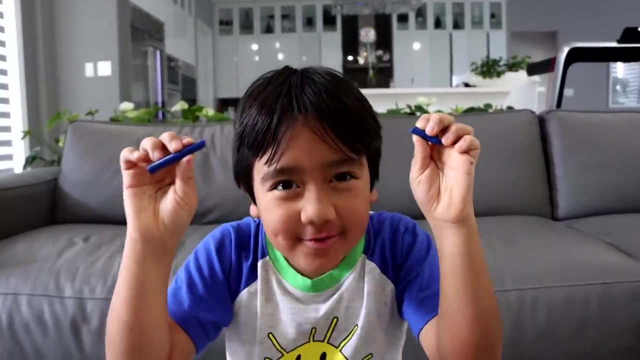 Here And here. Look, My rainbow is done. Well, other examples of physical change is crumbled paper. It's crumbled, but it's still paper. Score And Whoa, Oh no, My crayon broke. Well, that's okay. 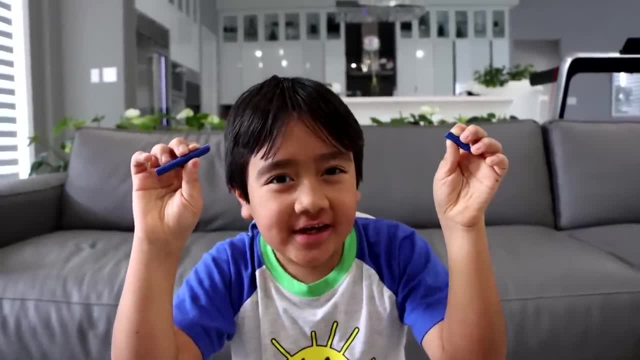 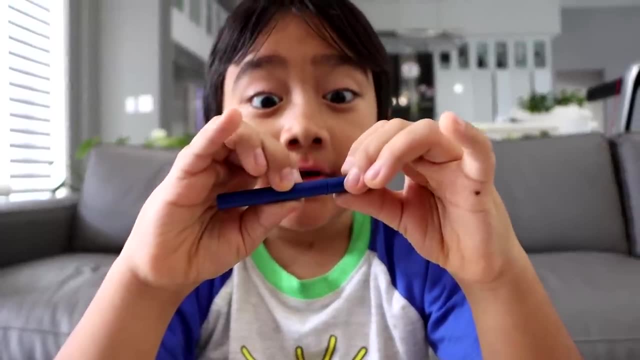 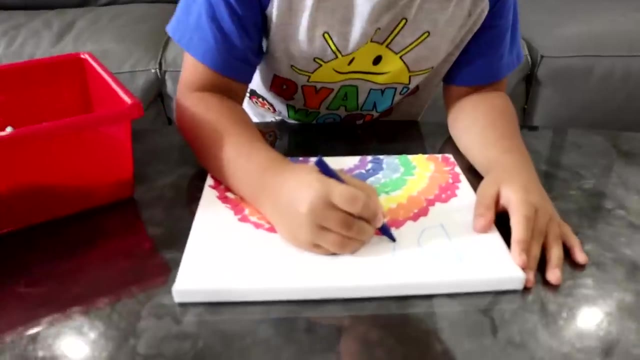 This is another good example of physical changes. It is broken, but it is still a crayon. I didn't create anything new. Good thing, I have more crayons and a lot more crayons. Okay, let's finish it up, And. 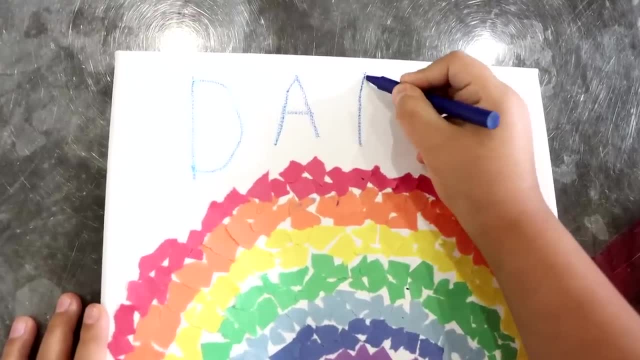 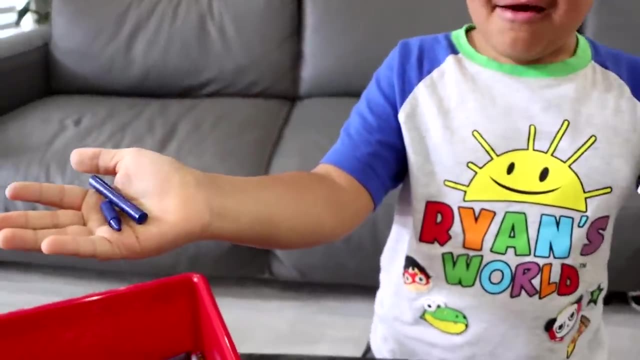 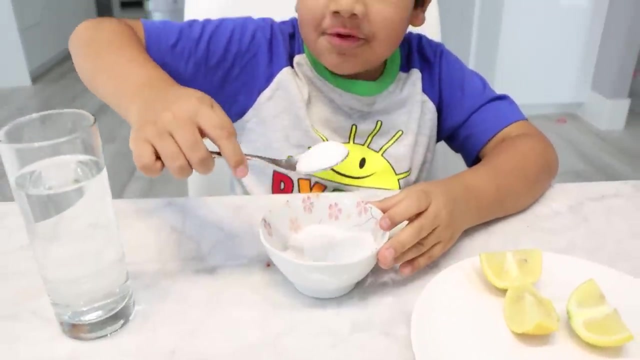 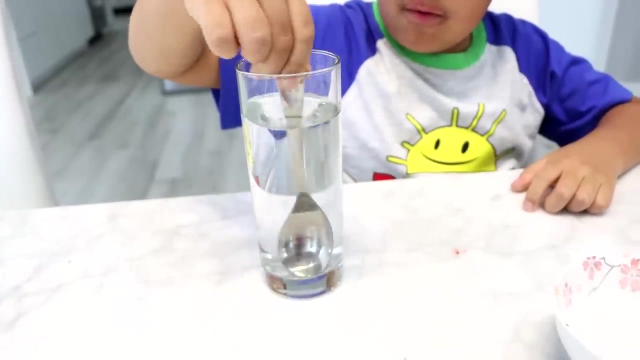 D. Oh Look, I finished, But Oh no, Not again. Physical change. Now I'm gonna make my daddy some lemonade. I'm gonna add one spoon of sugar into the water. That's a lot. This is an example of physical change, because I didn't create anything new. 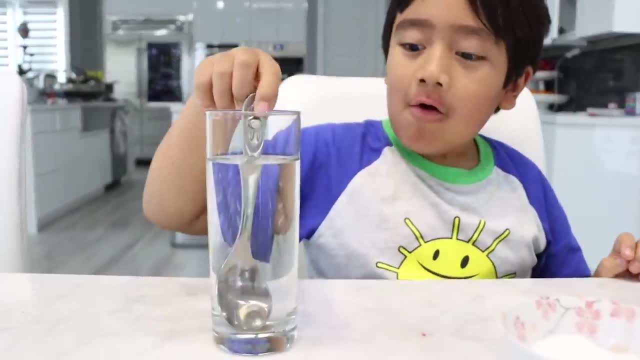 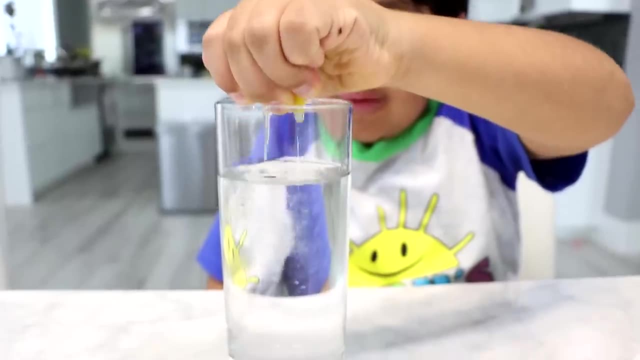 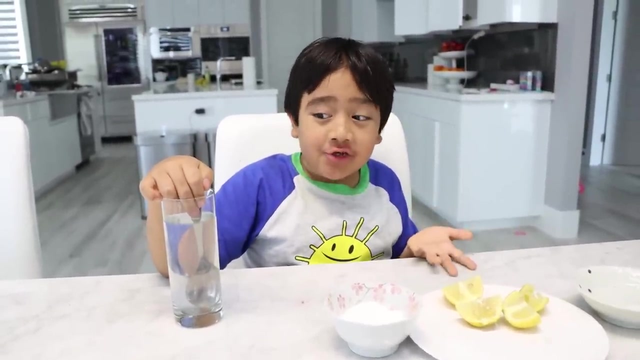 It's just sugar dissolved in water. Now let's add some lemons- Ooh, lemons. Now let's stir. This is also a physical change, because there's lemon juice mixing with the water. Now let's add in some ice. 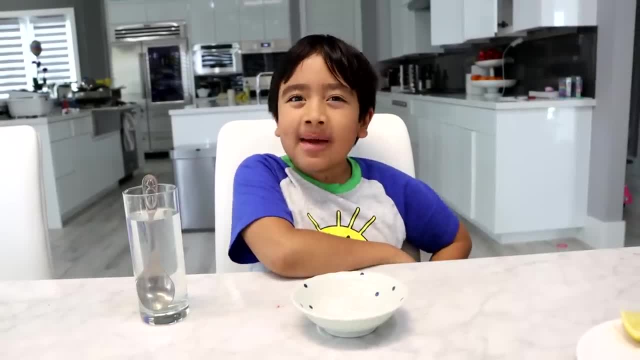 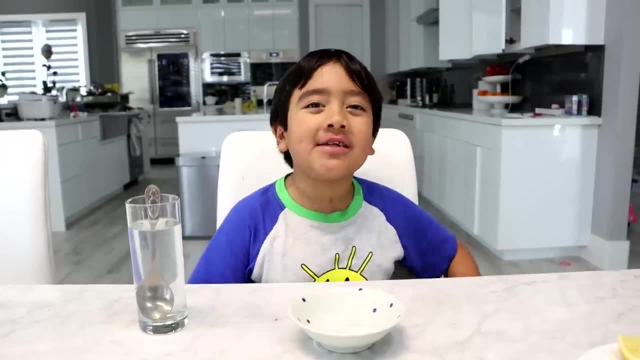 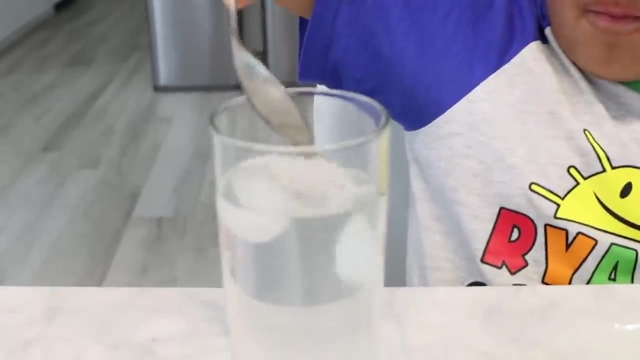 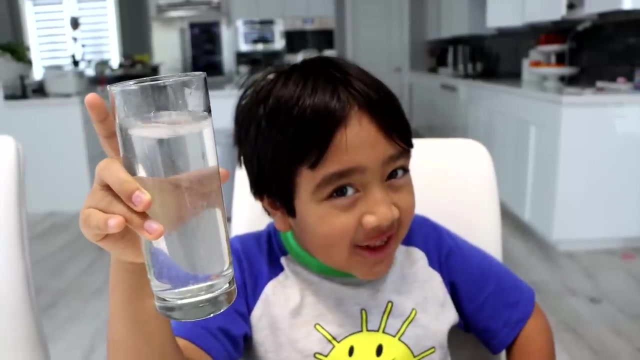 Wait, look, The ice melted. But this is also another good example of physical change. The ice did melt, but it's still water, water. So no chemical reaction takes place. Now let's add in some melted ice. Hopefully Daddy will enjoy this. Some nice lemonade, Physical change. Now I'm going to make a chocolate. 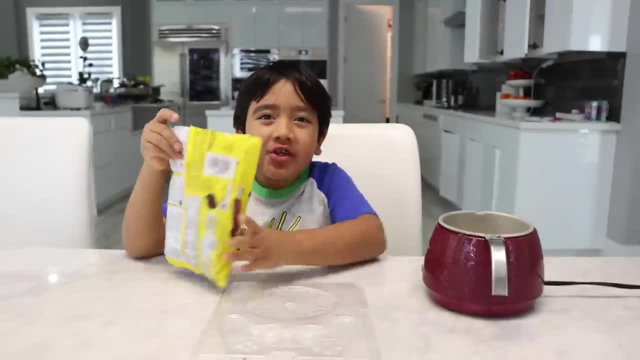 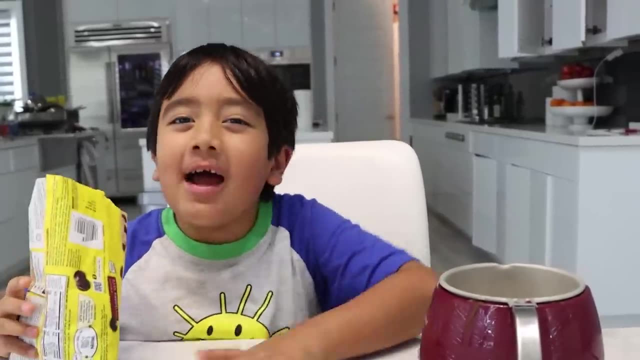 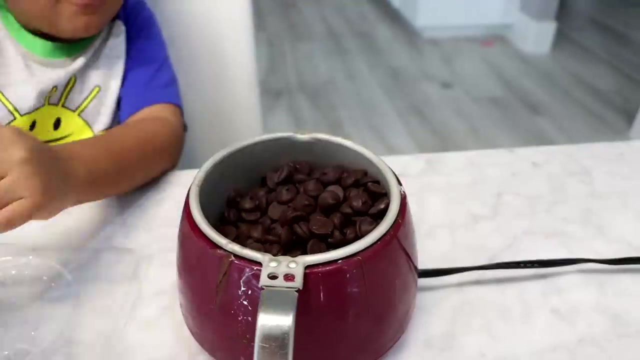 controller for my dad And I'm going to melt the chocolate. Let's do it, Wait. But before you do it you have to ask the parent for help, And I have money. Hi, Go ahead, It's a lot of chocolate. This is also another good example for physical change. It is still chocolate. 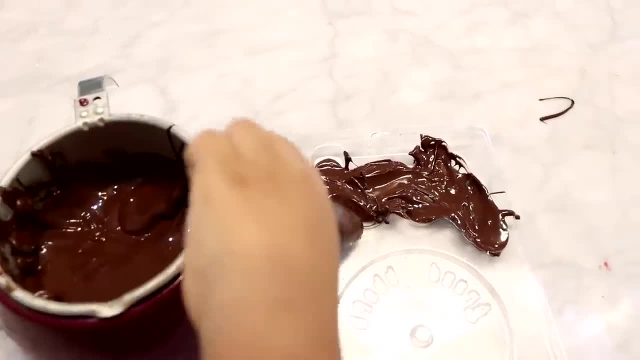 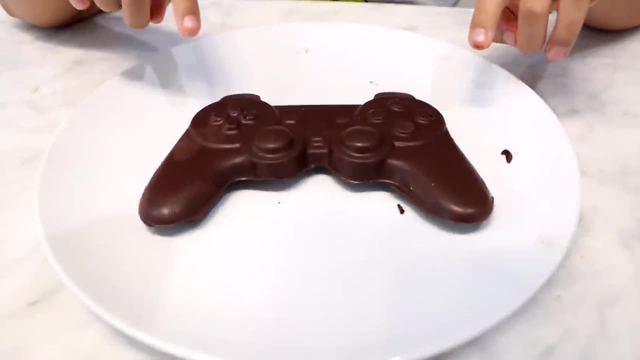 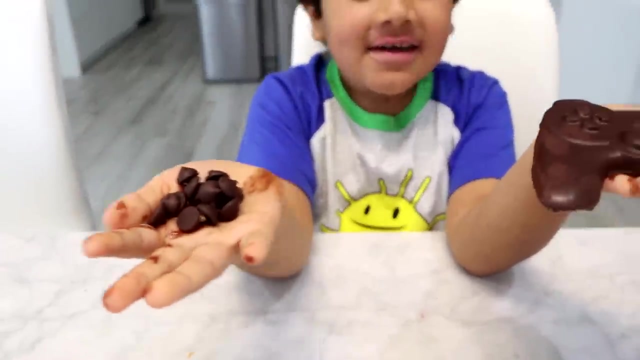 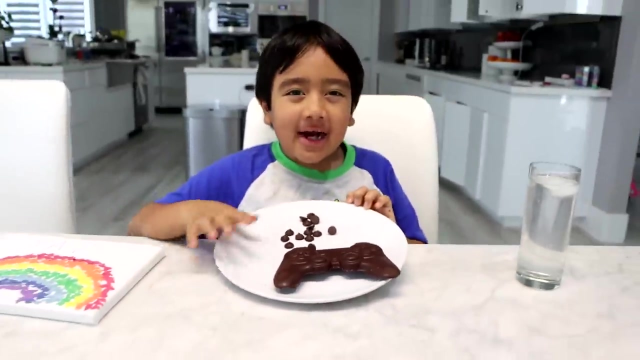 but it's melted chocolate. Look guys, my chocolate remote is done. The chocolate piece physically changed from this to this. I didn't create anything new. It's still chocolate, but looks different. Well, I'm going to call Daddy for his first surprise. Daddy, What's? 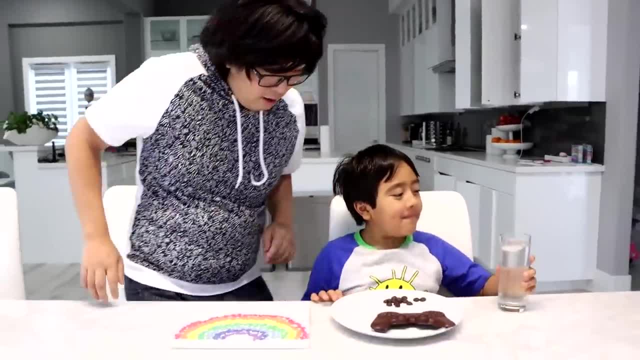 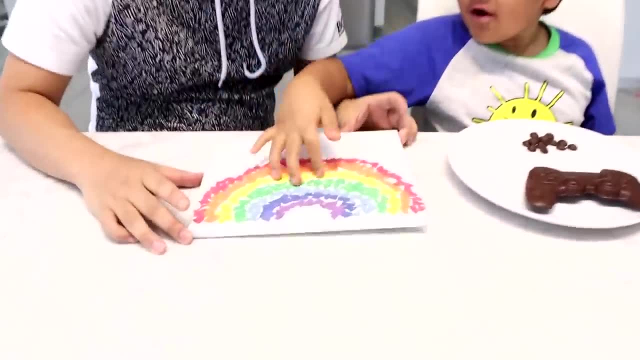 up Ryan. Hi, Mommy, What is this? Well, I got some lemonade, a chocolate controller and chocolate and also a rainbow that says Dad, Wow, is that for me? Now, what's the location? Happily ever after. 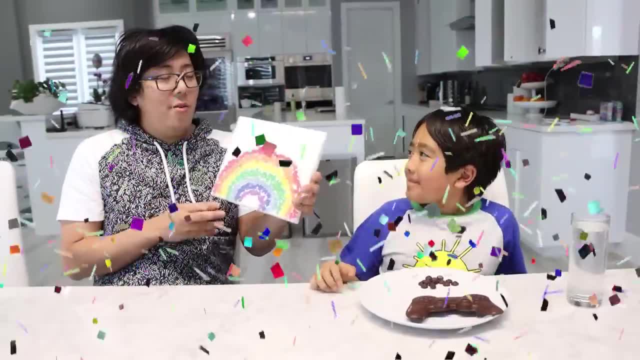 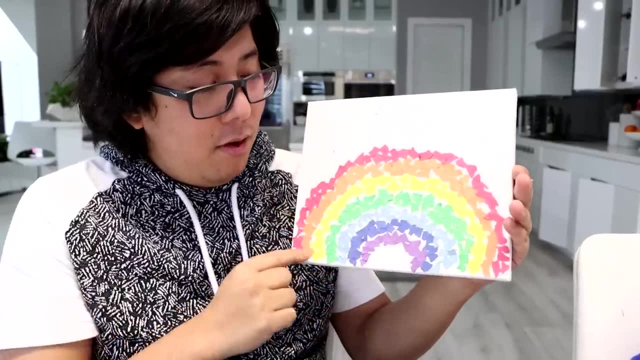 Happy birthday. Oh, thank you. Yeah, I love my birthday. Thank you, Ryan, Love this rainbow. Look at that. I like how you tear it and you get like paper pieces and then put it together like a rainbow. That's right, Daddy, Physical change. I tear the piece of paper up, but 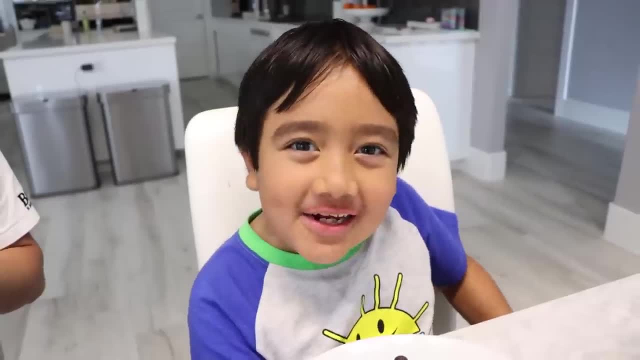 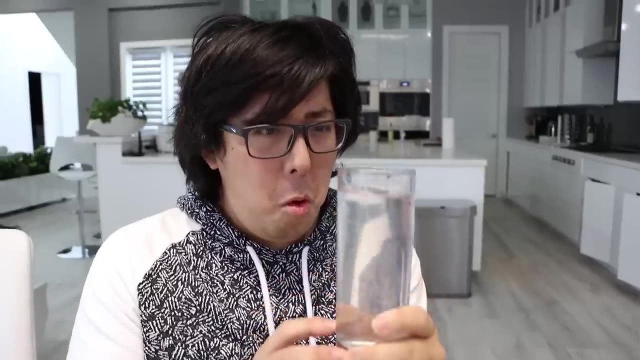 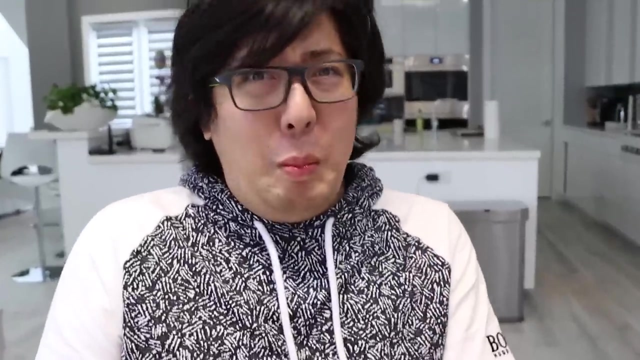 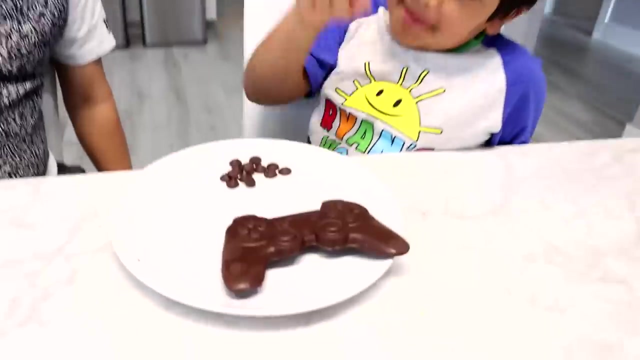 it's still paper. Physical. what Physical change? Well, hey, Daddy, want to try this lemonade. Oh, lemonade. Yeah, It's a homemade lemonade. You made it, Yeah, yeah, Oh good, Oh, it's super sour. Ryan, What about my physical change to remote controller? that's definitely. 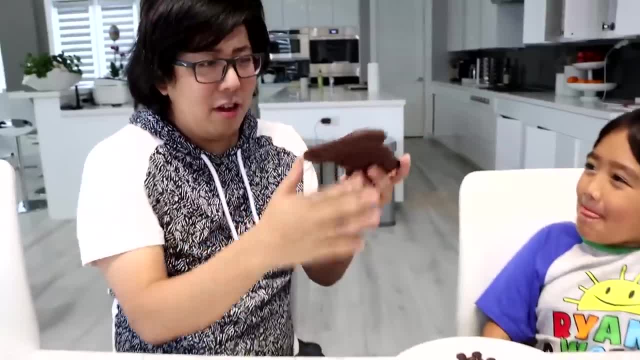 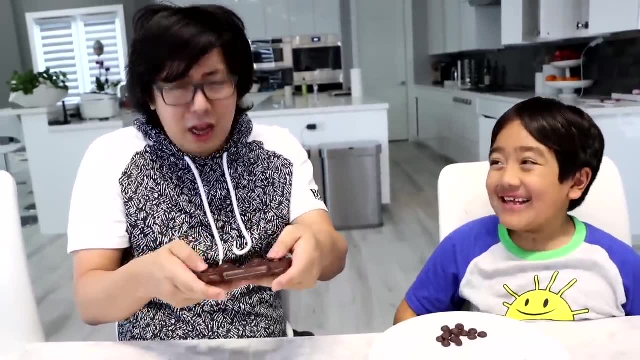 not chocolate. Whoa, yeah, it does look like a controller, right. Can I actually use it in my gaming? Yeah, yeah, yeah, yeah, yeah, Are you sure? I don't think the buttons are working? Wait, it's melting. It's chocolate, Ryan. 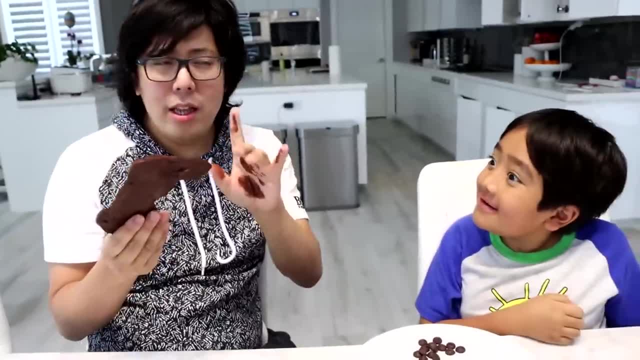 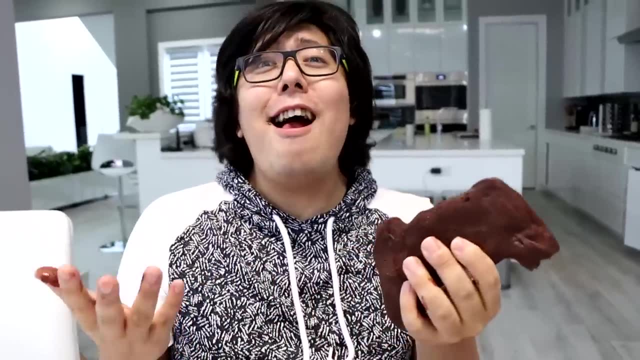 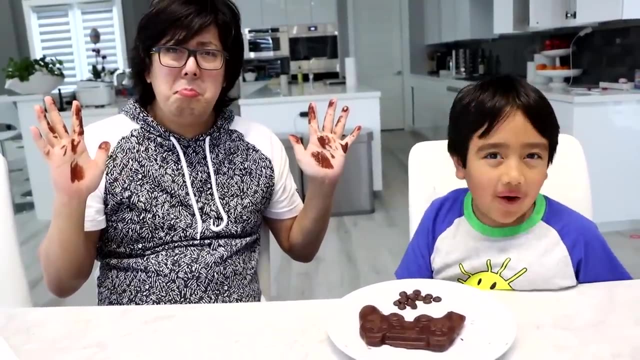 Look at my hand, But let me taste it first. I don't know, until I taste it It could be something else. right, It might not be chocolate. Let's see, It is chocolate. Yeah, That is tasty. I have more surprises for you later, Daddy, But first more physical changes Is. 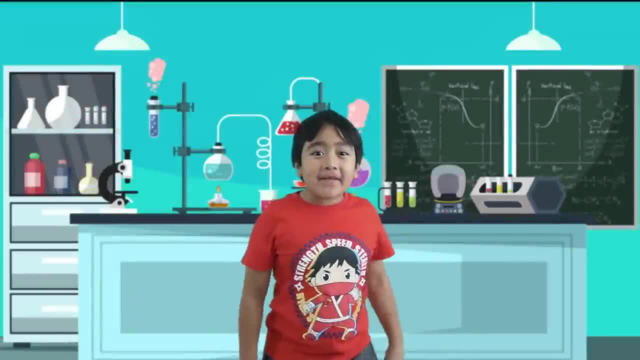 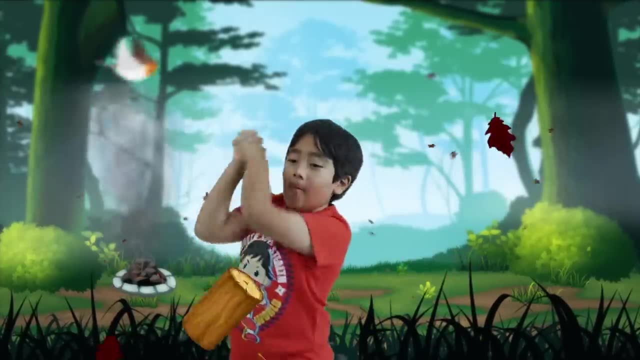 this physical change too. Remember, a physical change is when no new substance is formed. It just looks different whenever you're in the game. Yeah, yeah, yeah, yeah, yeah, yeah. When you're cutting wood, it may look different because you cut into pieces, but it's still. 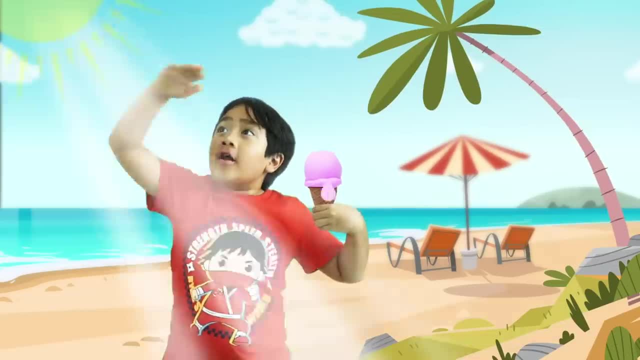 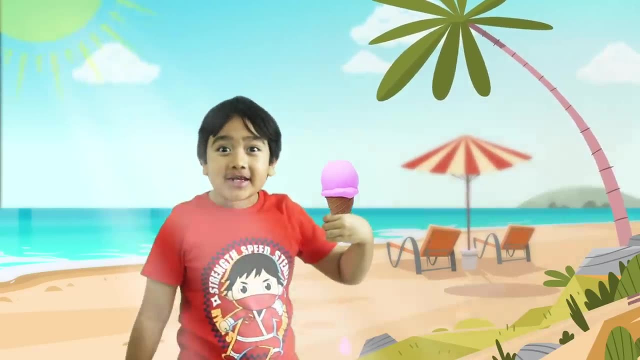 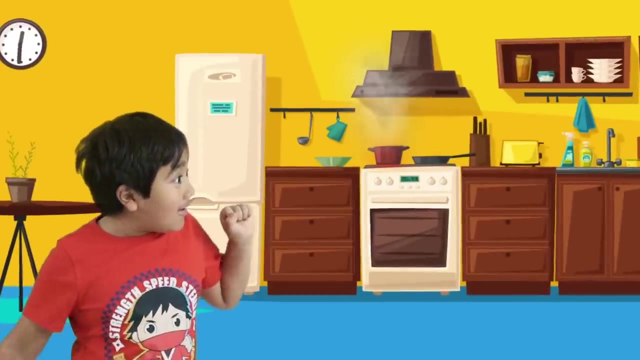 wood. Physical change. On a hot sunny day, your ice cream might melt, but it's still ice cream. It's just melted ice cream. Physical change Whenever water is boiling on a stove: ah, it's hot. The liquid changes into a gas, but it's still H2O. 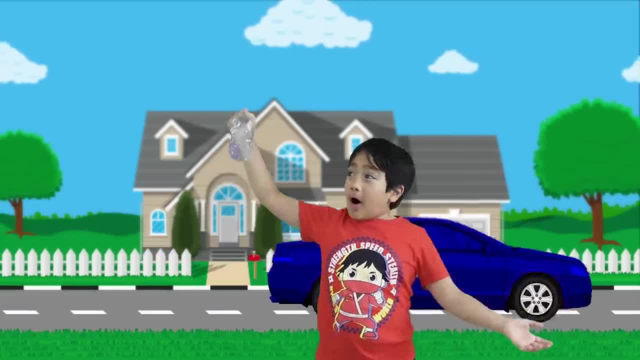 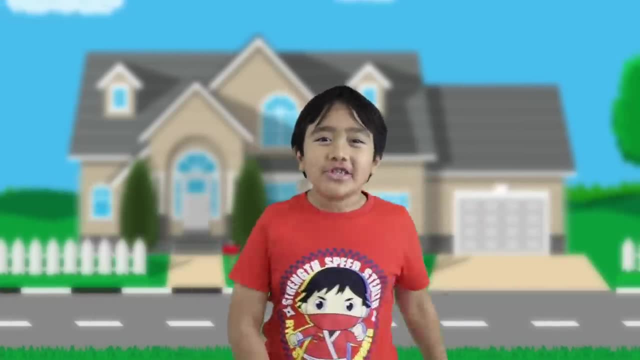 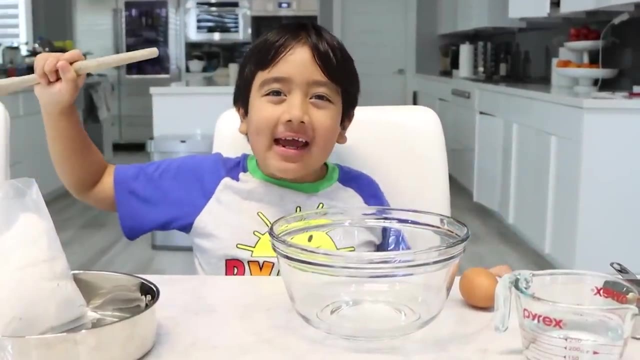 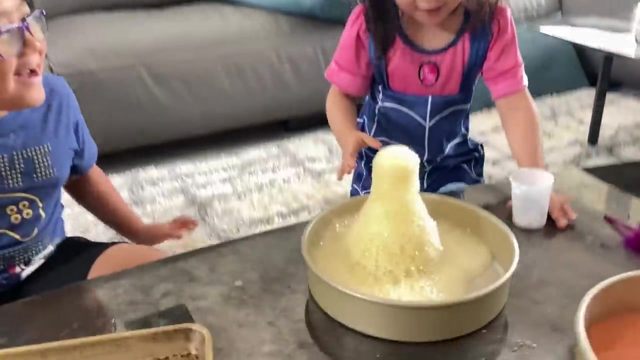 Physical change. Whenever you crush a water bottle, it's still a water bottle, It's just crushed Physical change. Now that we learned all about physical change, let's learn about chemical change. A chemical change is when a substance is formed, For example the class. 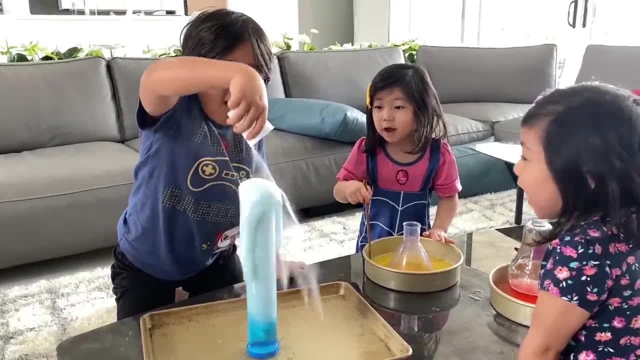 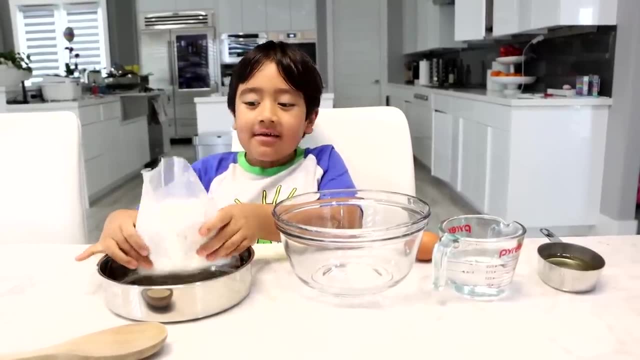 of baking soda and vinegar: science experiments. This experiment, we're going to learn about chemical change. When a substance is formed, it creates bubbles, which is the carbon dioxide gas that's being released. Now I'm baking my teddy a cake First. I need flour Next. 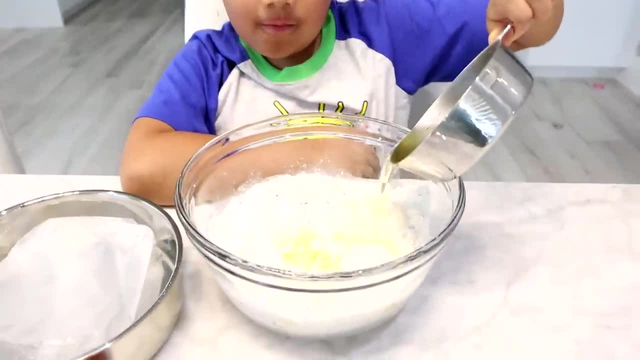 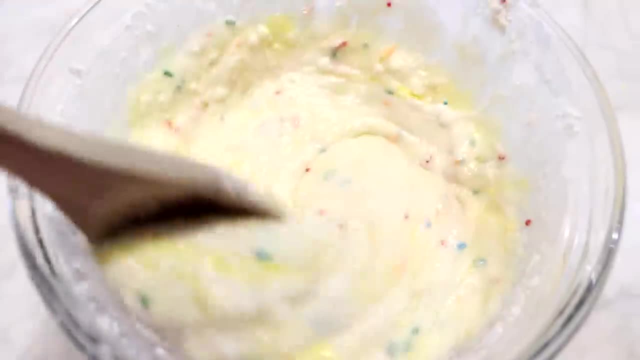 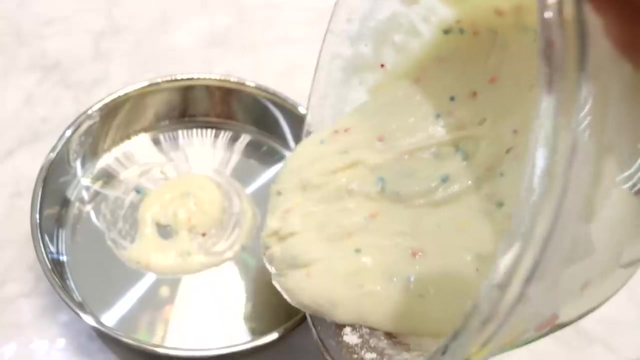 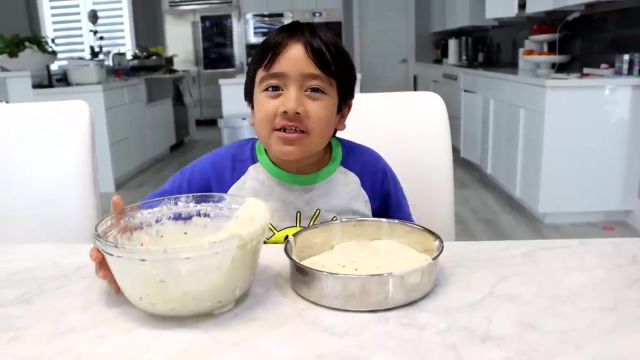 water and then vegetable oil. Crack the egg, Next add the cake. This is a physical change, because we haven't created anything yet. Put it into the pan. Ooh, Okay, let's bake the cake for Daddy. Don't forget to ask the grownup for help to put. 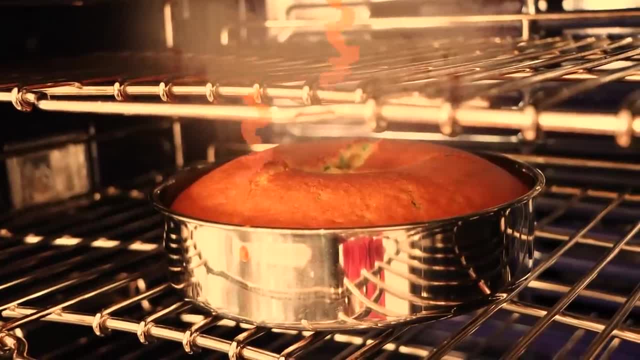 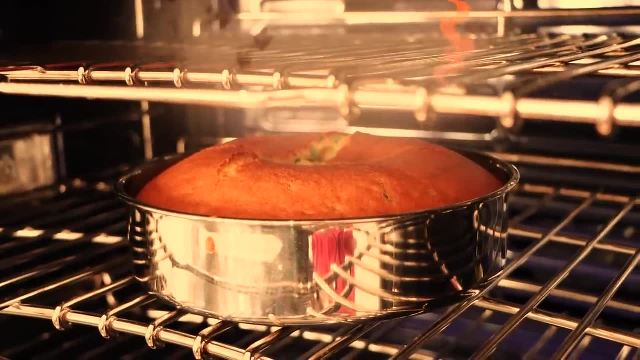 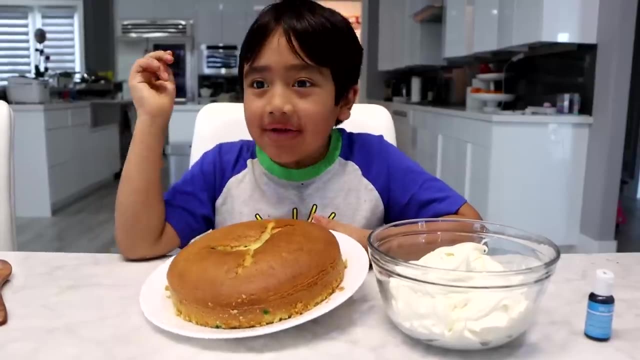 the cake into the oven. As you bake the cake, it creates a chemical reaction. The ooey gooey batter changes into a fluffy, yummy cake. The heat from the oven causes protein from the egg to change and make the cake firm. Guys, look, the cake is done And this is. 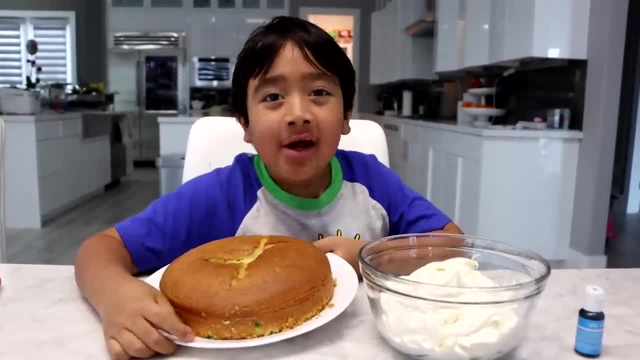 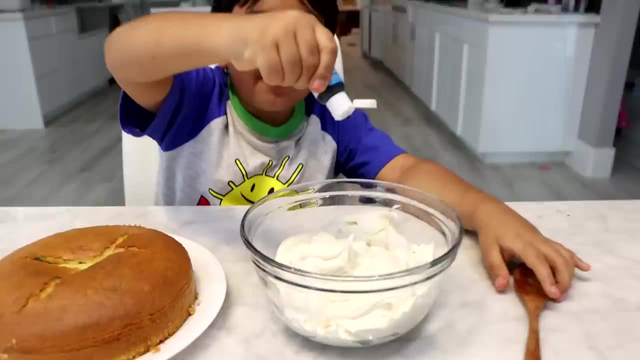 a good example of a physical change. Okay, let's bake the cake for Daddy. Don't forget to ask Daddy, This is a chemical change because I created something new: a yummy, delicious cake. Now for the frosting. I'm going to color it blue, Guys. quick question, do you think? 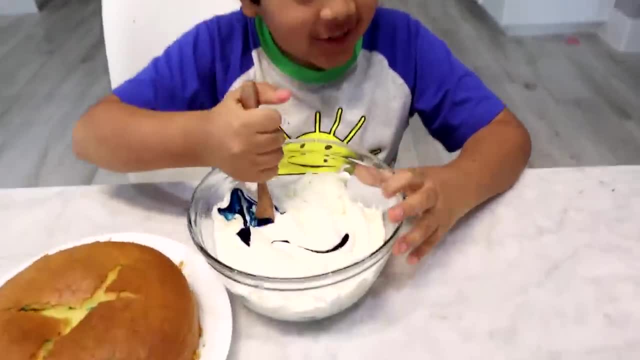 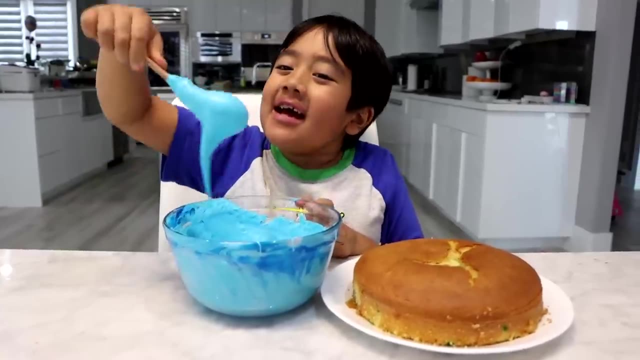 this is a chemical change or a physical change. Look, guys, It's turning blue. Did you guys guess it? It's a physical change because it's still frosting, but it's blue because it's a chemical change. Guys, look, It's turning blue, exactly like the color I just painted. 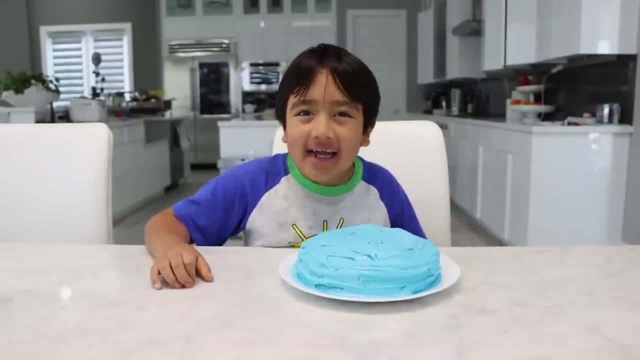 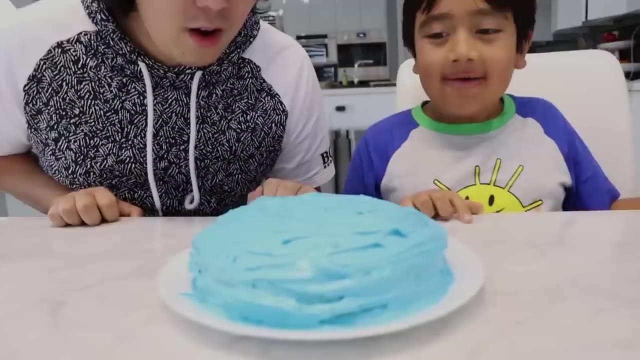 Can you guess what this is? It's a physical change because it's still frosting. but it's frosting. the cake is ready. let's call daddy. daddy, what is it? happy birthday, daddy. i made you a cake. whoa, that looks so delicious. thank you, ryan, and candles. 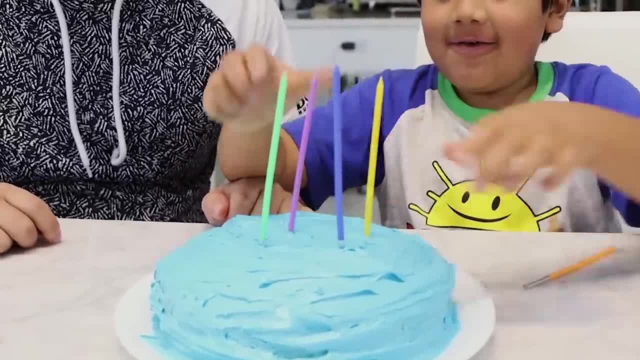 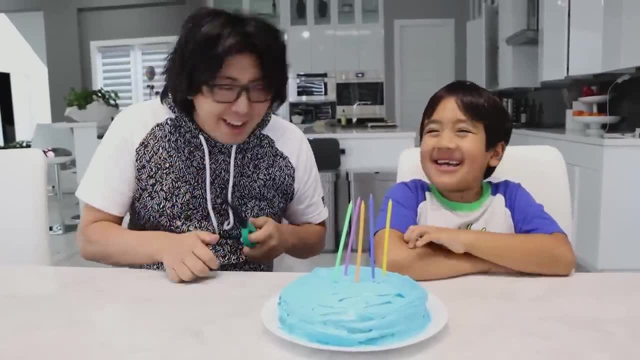 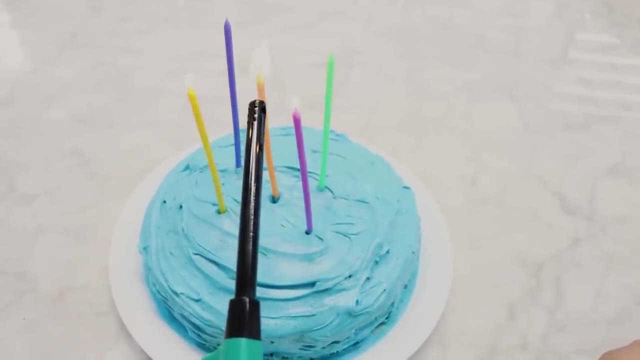 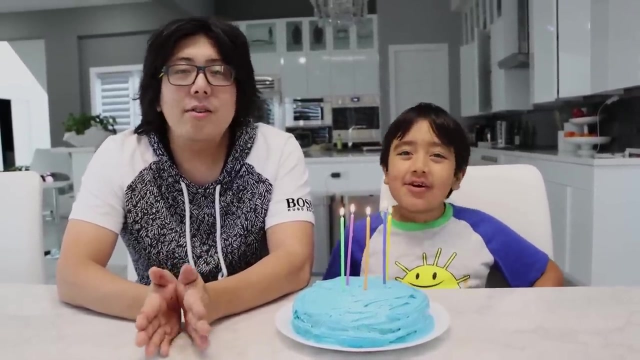 one, two, three, four and five, five candles. yeah, i'm five years old. yeah, guys, remember, always ask parents for help when you light up the fire on the candle. let's sing: my dad, happy birthday, happy birthday to you. happy birthday to you. happy birthday, dear daddy. happy birthday to me. 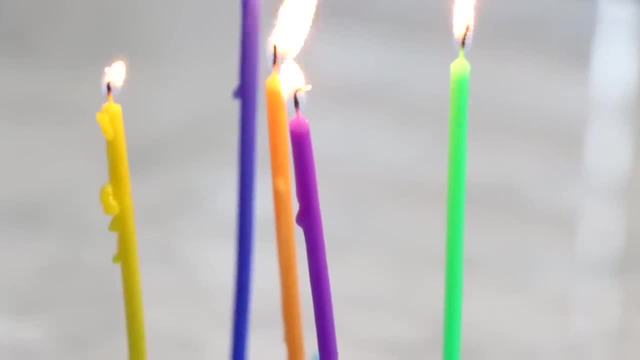 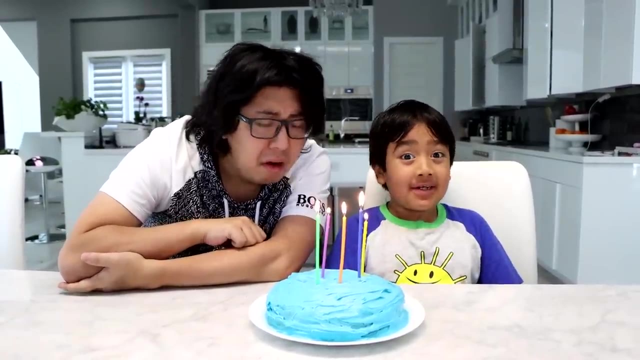 thank you, ryan whoa, all right, it's melting. you better hurry up and blow it away. look, daddy, i have a question for you. is a candle that's melting a physical change or a chemical change? hmm, i think it's physical change. it's still a candle. 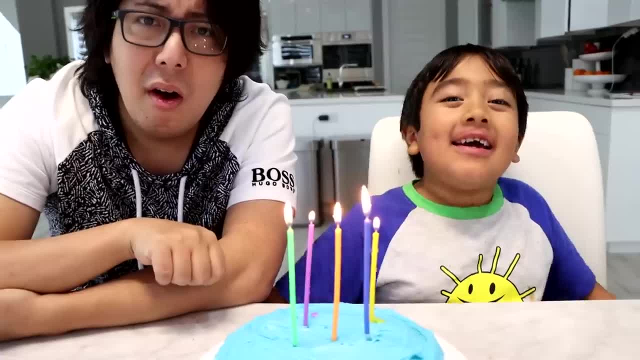 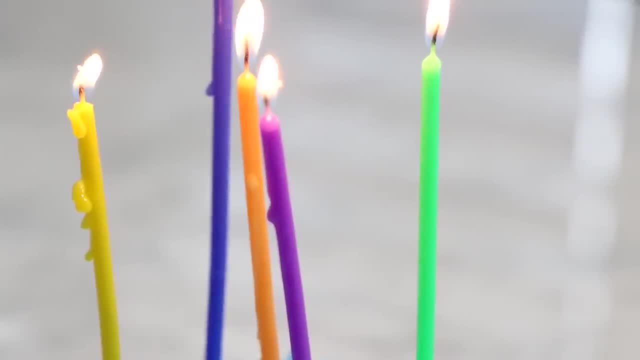 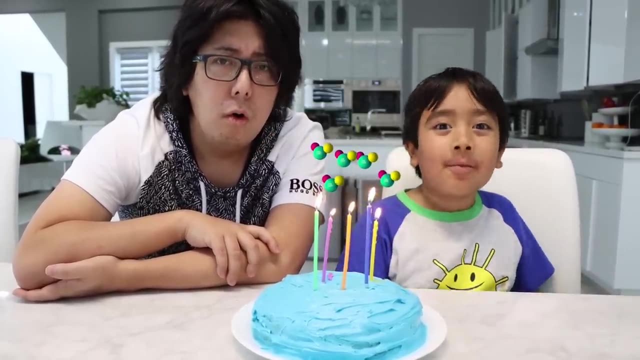 right, it's melting, but it's still a candle. yeah, it is a physical change, because the wax is melting, but it's still wax that's melting. but it's also a chemical change, because whenever you're burning the candle, it creates carbon dioxide and releases water vapor. what 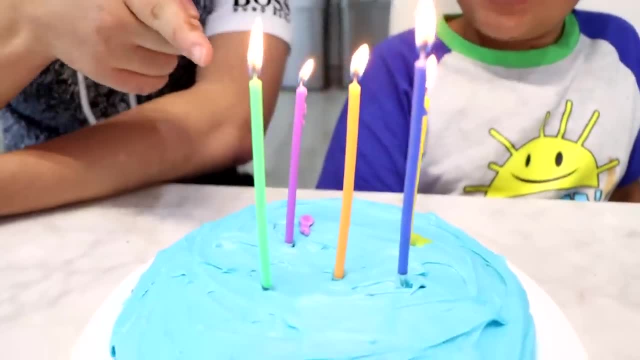 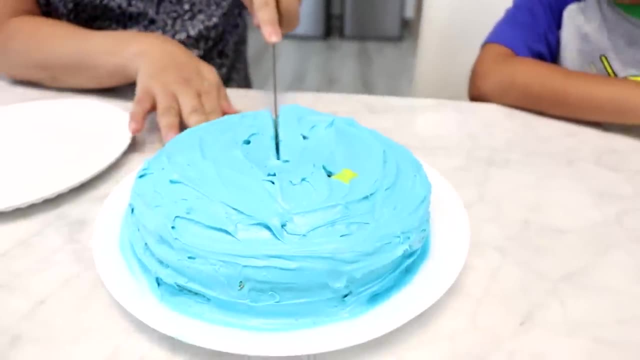 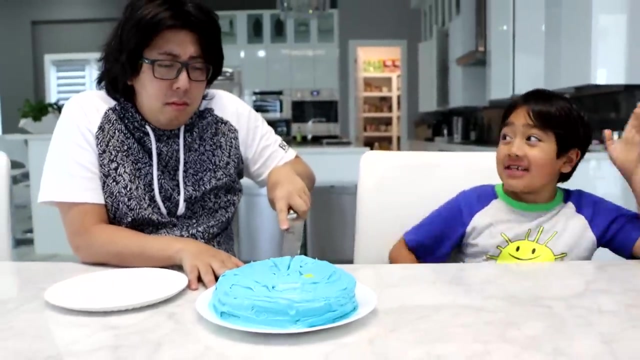 i don't know, know that. but hey, just hurry up. can i blow it? now it's melting. yeah, blow it up, i'm gonna get a big slice for myself, a big slice, and, daddy, whenever you cut the cake, is that a physical change or a chemical change? a physical 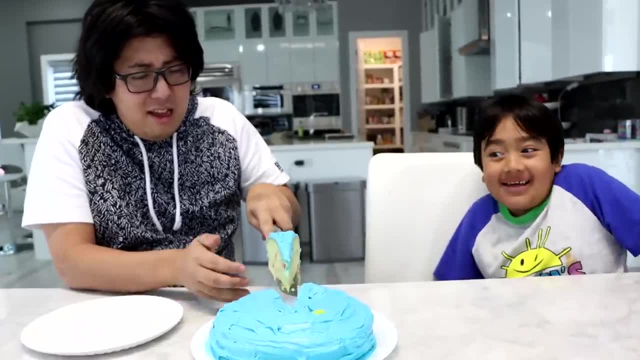 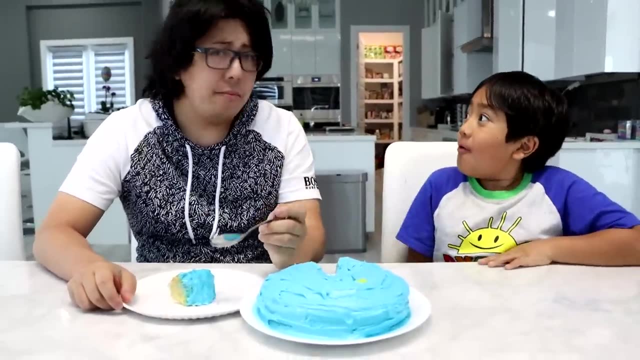 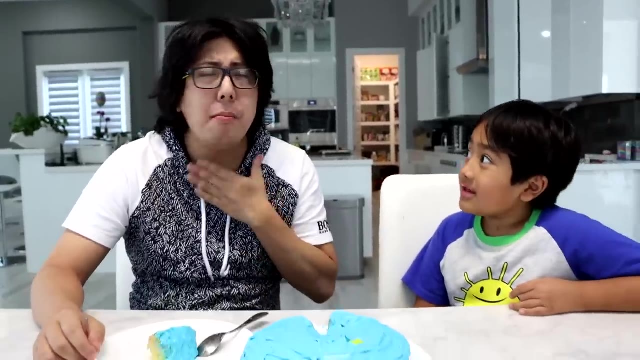 change. yeah, it's a physical change, because it's still cake and it's physically looking perfect. yeah, yeah, like i could just put a very, very, very big, big piece like this here, sort of like. so, yeah, it makes a very big, bigger one. oh, come on, get it out alright. 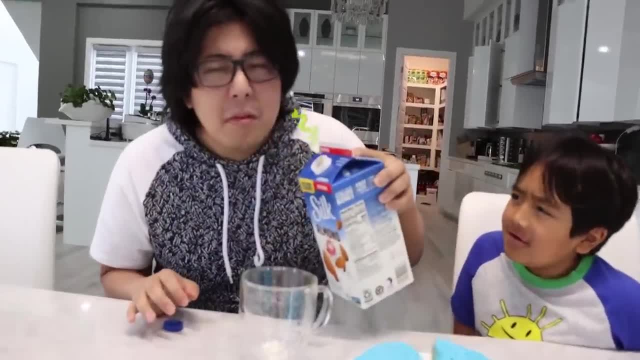 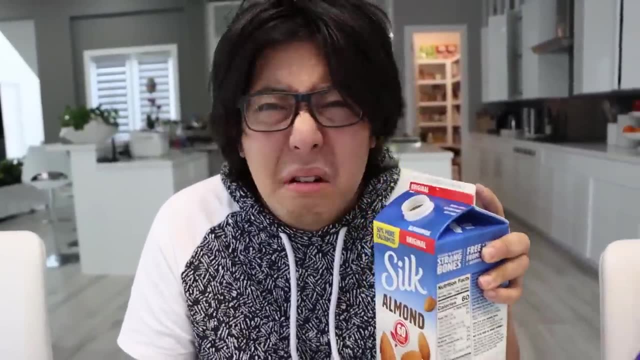 so there's the card that i brought. hmm, could that be removed? yeah, but you know what? i need some milk. let me go get some milk. okay, yeah, i can't have a cake without milk. yeah, all right, wait, i smell something funny. oh yeah, ah, i think this milk has expired. it smells sour. low daddy, is expired, soured, and it's most amazing in reality. 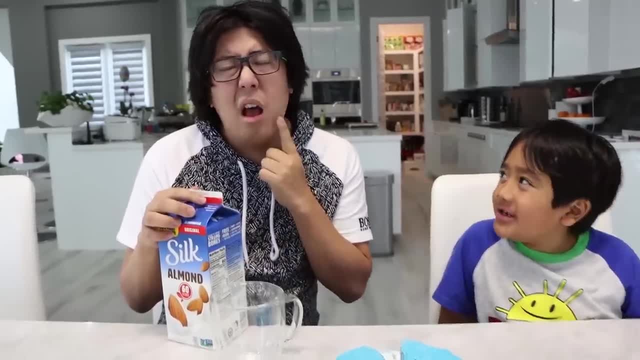 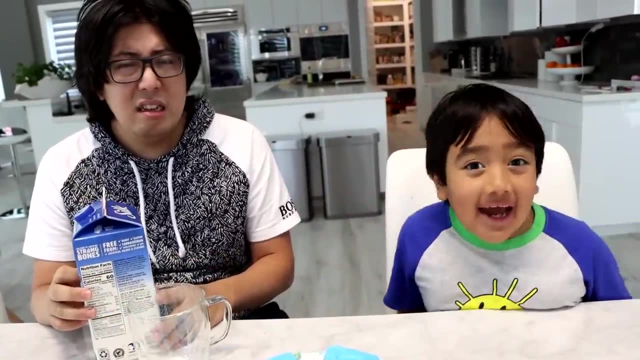 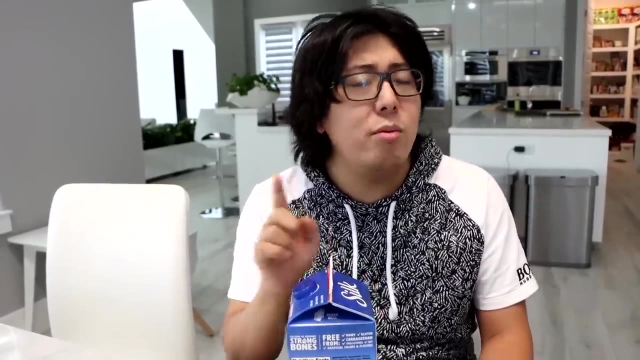 Will milk a physical change or a chemical change? Uh, chemical change. Yeah, that's right, Because the bacteria in the milk creates lactic acid, which causes the milk to be sour. Oh, something new was created. That's why it's a chemical change. 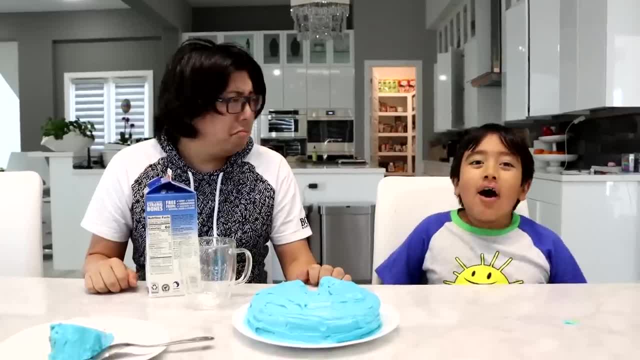 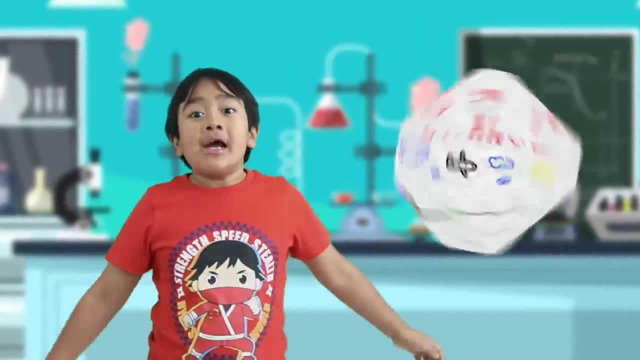 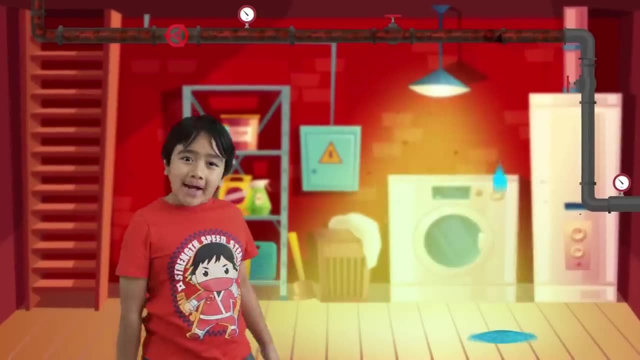 But hey, can I just get a milk without chemical change? Okay guys, here's some more fun examples of chemical changes. Remember, a chemical change is when something new was formed or created. Iron rusting is an example of a chemical change.